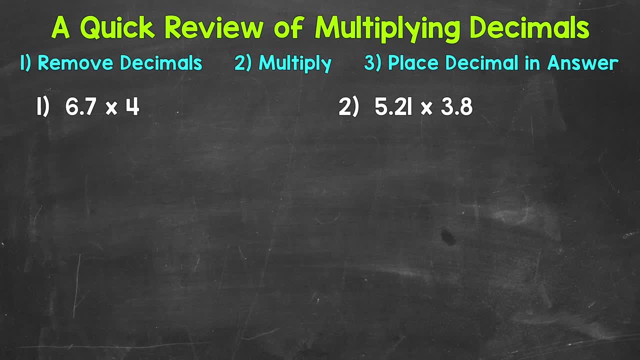 Now the first thing that we're going to do when we have a multiplication problem that involves decimals, we're going to remove any decimals within the problem, So we're going to multiply just like we would if we had whole numbers. Let's set this up and rewrite number 1 as 6.. 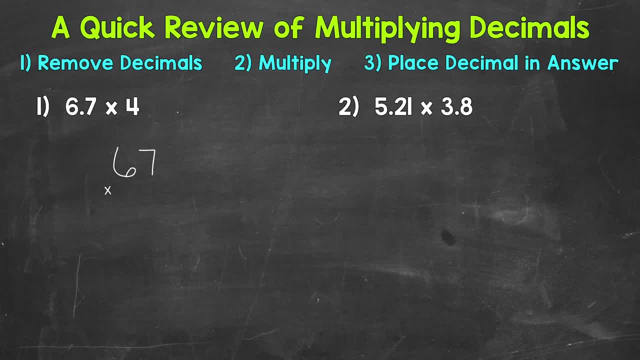 67 times 4.. So again, remove any decimals. We're going to worry about placing the decimal in our answer once we multiply. So once we remove the decimals, we can multiply. So we'll start with 4 times 7, which is 28.. 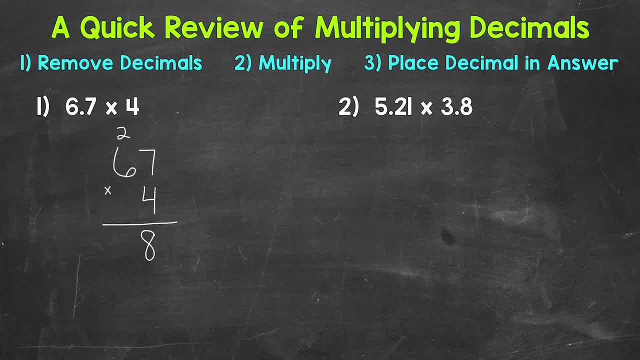 So carry that 2.. And then we have 4 times 6,, which is 24.. Plus that 2 is 28.. So we have 4 times 6,, which is 26.. Now we're done multiplying, so we can place our decimal in our answer. 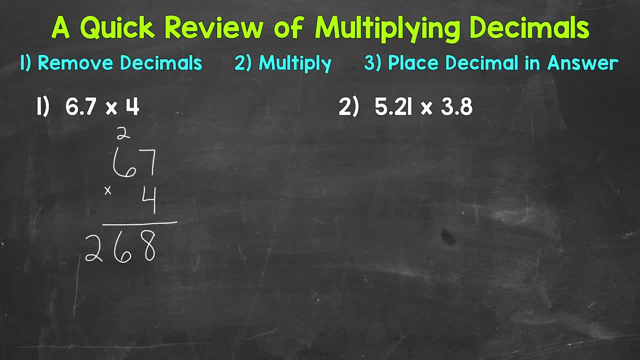 So we take a look at the original problem and see how many digits are behind or are to the right of a decimal. Well, 1. We have this 7 right here, to the right of a decimal. So our answer is going to have one digit to the right or behind the decimal. 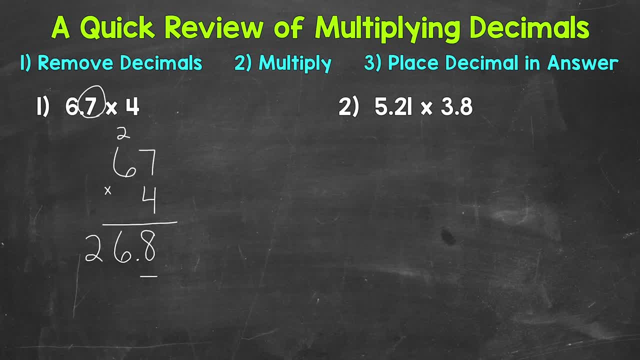 So one digit would be this: 8.. So we can place our decimal in between the 6 and the 8.. Our final answer: 26 and 8 tenths. Let's move on to number 2, where we have 5 and 21 hundredths times 3 and 8 tenths. 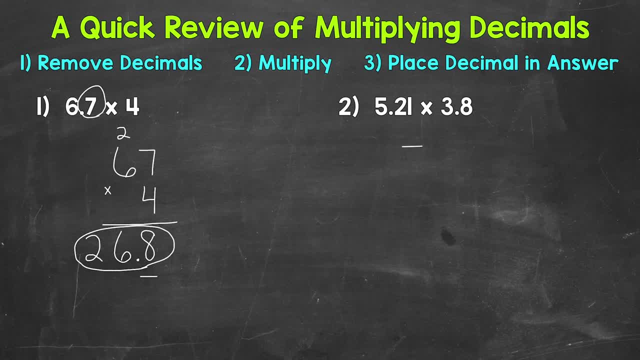 So let's remove the decimals and rewrite this problem. So: 521 times 38.. Now we're ready to multiply. So 8 times 1 is 8.. 8 times 2 is 16.. Put our 6.. Carry the 1.. 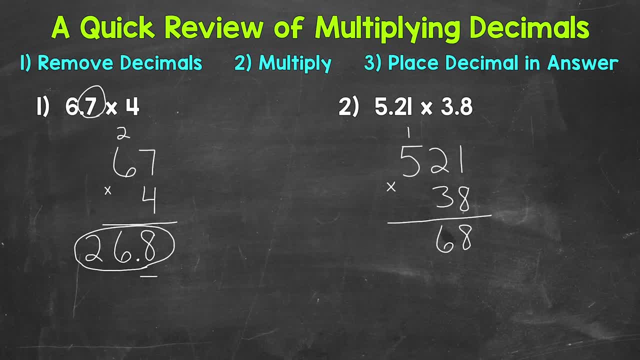 And then 8 times 5 is 40. Plus that 1 is 41. So we are done with the 8. And we are done with this carried 1.. So we're going to move over to the 3.. We're moving one place value to the left. 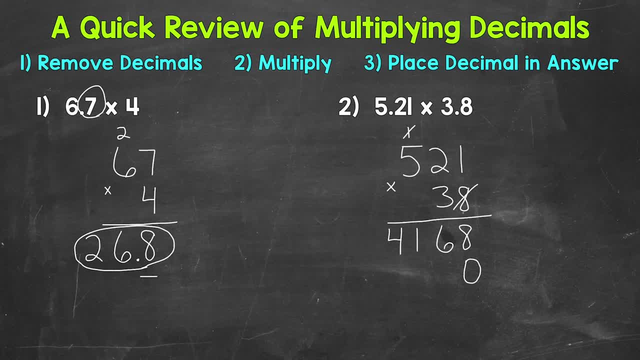 So we need our placeholder 0 here. And now we multiply, starting with 3 times 1,, which is 3.. 3 times 2 is 6.. And then 3 times 5 is 15.. Now we add: 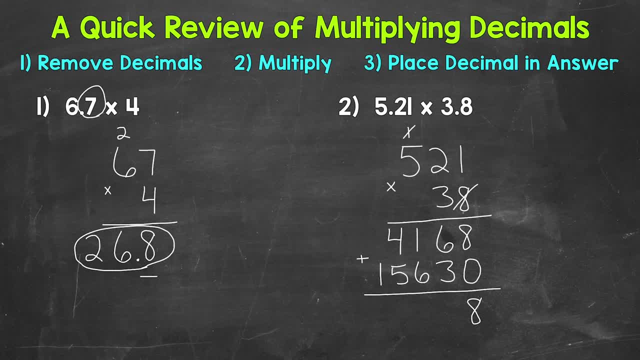 So 8 plus 0 is 8.. 6 plus 3 is 9.. 1 plus 6 is 7.. 4 plus 5 is 9.. And then we have a 1.. So once we get to this point, we look at our original problem and see how many digits are to the right or are behind a decimal. 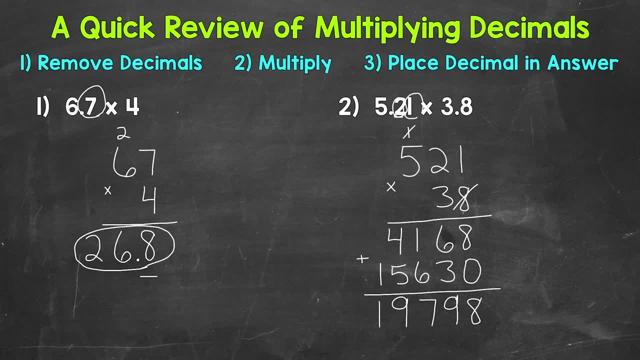 Well, this 2 would be 1.. This 1 would be 2. And then this 8 would be 3.. So we have 1,, 2,, 3 digits behind or to the right of a decimal. So our answer: 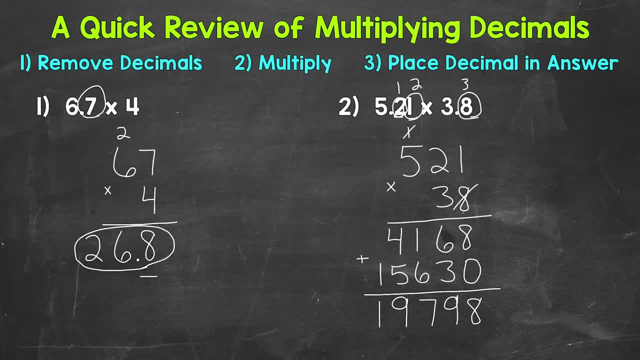 Needs 3 digits to the right of the decimal. So we have 1,, 2,, 3 digits. Our decimal is going to go between the 9 and the 7.. Our final answer: 19 and 798 thousandths. 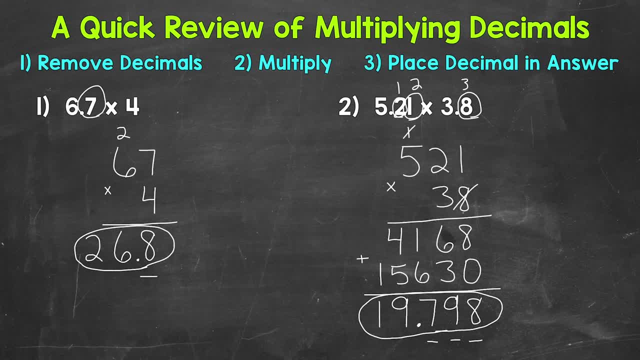 So there you have it. There's a quick review of multiplying decimals. Remove the decimals, Multiply as you normally would with whole numbers And then Place your decimal in the answer. Look at the original problem, See how many digits are to the right or are behind a decimal. 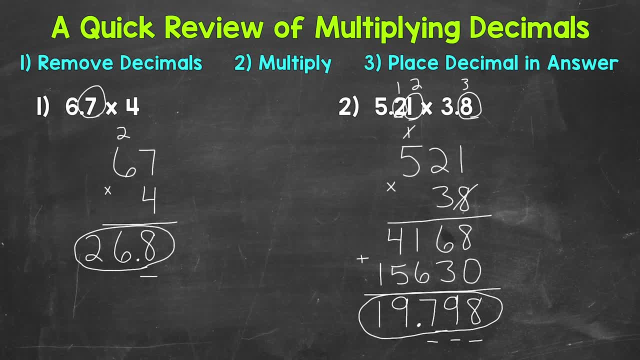 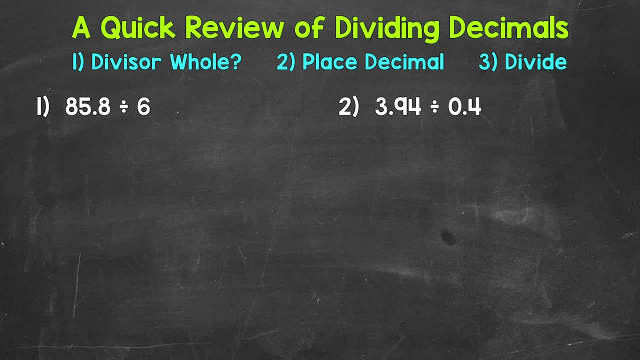 And then your answer is going to match that. Let's move on to division. Here are our examples of dividing decimals. Let's jump into number 1, where we have 85 and 8 tenths divided by 6.. Now, the first thing that we're going to do, 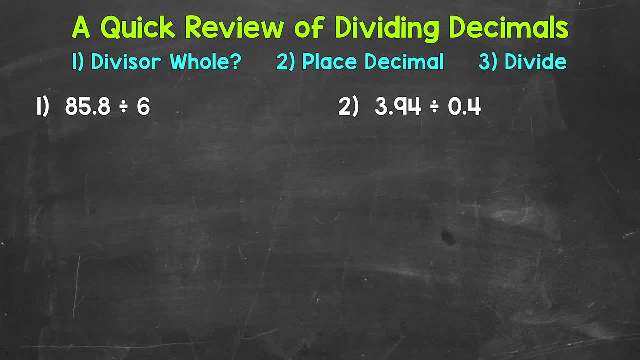 We're going to set the problem up And place it. Place our decimal For number 1. we have 85 and 8 tenths for our dividend. That's the number we are dividing, So it goes under our division bar. So let's write out 85 and 8 tenths. 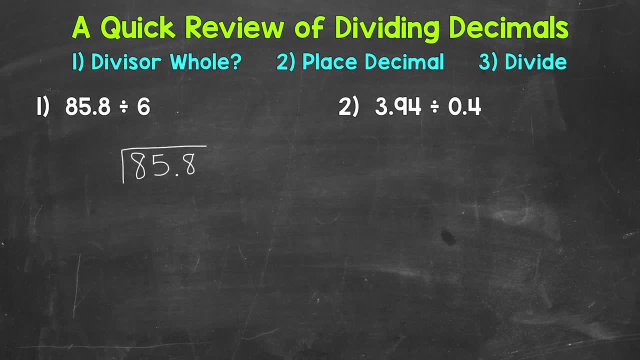 And then we are dividing by our divisor of 6.. So the divisor is the number we are dividing by. Once we get to this point and we are set up, We have a very important question: Is our divisor a whole number? If yes, our decimal goes straight up into our answer. 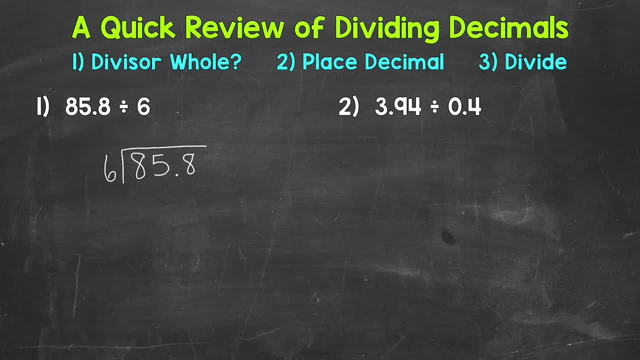 For number 1, our divisor is whole. We have a 6. So let's bring that decimal straight up into our answer. So our decimal is placed and we are ready to move on. Now I do want to mention For number 2. we will see what happens when we do not have a whole number for our divisor. 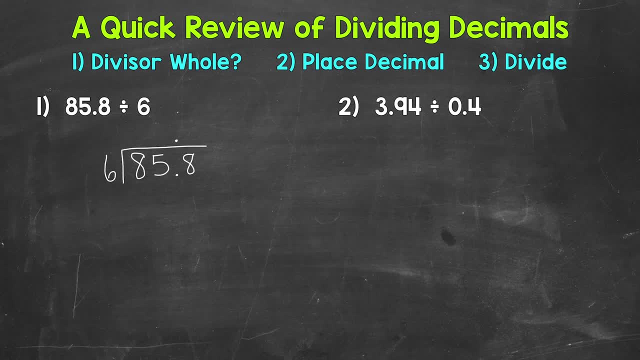 So once we bring that decimal straight up into our answer, We can divide as we normally would with whole numbers. So we're going to use the same division process that we use with whole numbers: Divide, Multiply, Subtract, Bring down, Repeat. 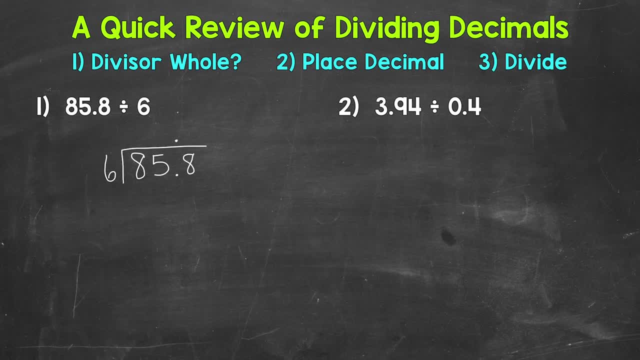 So let's start with divide. So we have 8 divided by 6. How many whole groups of 6 are there? 6 are in 8. Well, 1.. Then we multiply 1 times, 6 is 6.. 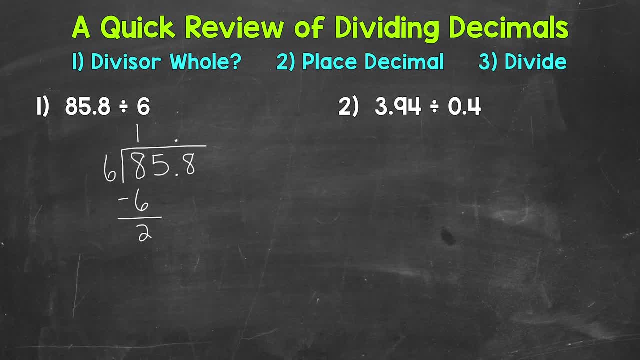 Subtract 8 minus 6 is 2.. And then we bring down, Now we repeat: So: divide 25 divided by 6. How many whole groups of 6 in 25?? Well, 4.. Multiply 4 times 6.. 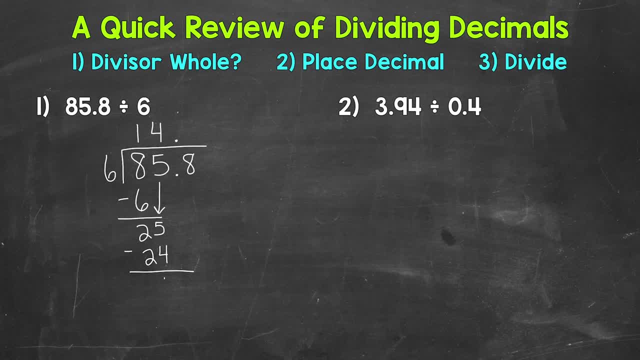 24. Subtract, We get 1. And then bring down our 8. So we repeat: now We go back to divide: 18 divided by 6. How many whole groups of 6 in 18?? 3. Multiply. 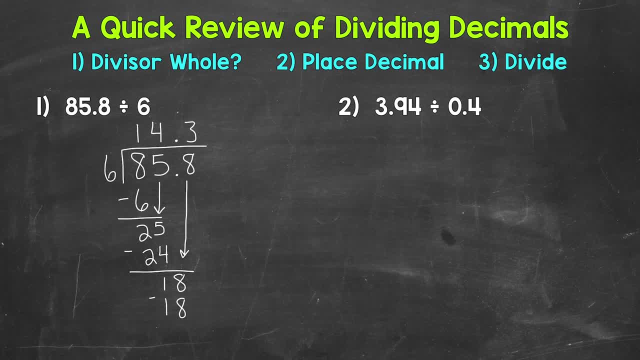 3 times 6 is 18.. Subtract: We get a nice clean cut 0 there And we are done. We went all the way to the end, All the way over to our furthest place value to the right. In the case of number 1, that's going to be the tenths place. 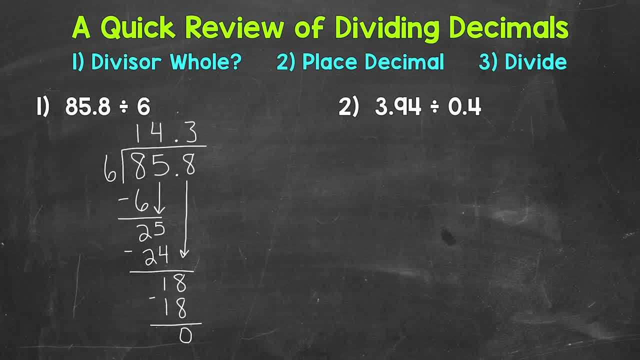 And then we get that clean cut 0, so we don't have anything left over. We do not need to continue the problem. Now for number 2. we'll see what happens once we go all the way over and we do not get that 0 there at the bottom once we subtract. 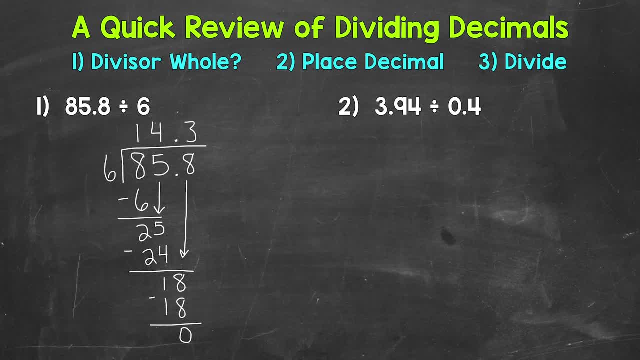 But for number 1 we are done. Our final answer: 14.. And 3 tenths. Let's move on to number 2, where we have 3 and 94 hundredths divided by 4 tenths. So we need to set this up. 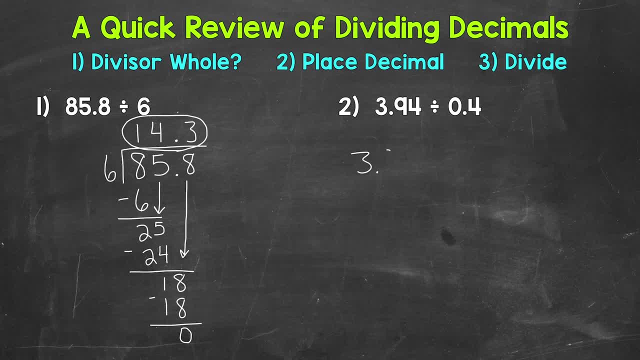 3 and 94 hundredths is our dividend, The number we are dividing, And we are dividing by 4 tenths. So once we're set up we need to see if our divisor is whole. Well, 4 tenths, We need to set a whole number. 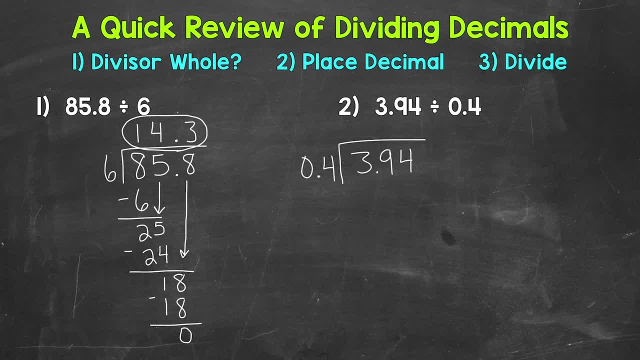 So we cannot bring the decimal straight up quite yet. If our divisor is not whole, we need to make it whole. Making the divisor a whole number gives us the ability to go through our division steps And it's going to place our decimal for us in our answer. 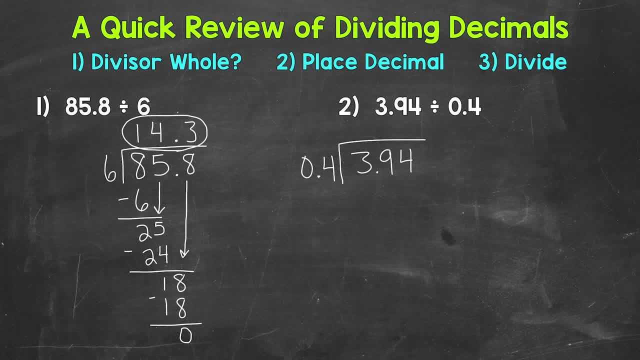 It's pretty cool how this works out. In order to make our divisor whole, we need to move the decimal once to the right, which means We are multiplying it by 10.. So let's move this decimal once to the right Now in order to keep this problem balanced. 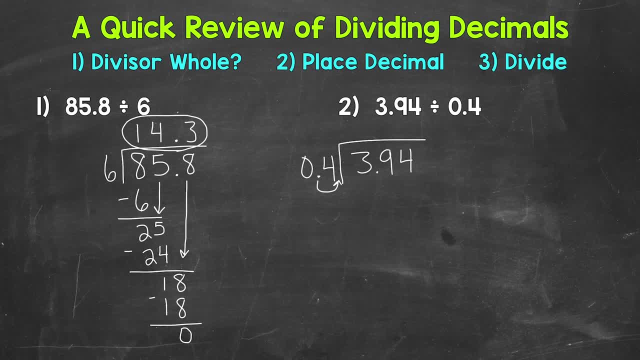 Whatever we do to the outside- The divisor, We must do to the inside- The dividend Again. This keeps the problem balanced and equivalent. Let's move the decimal once On the inside as well, So multiplying the dividend by 10 also. 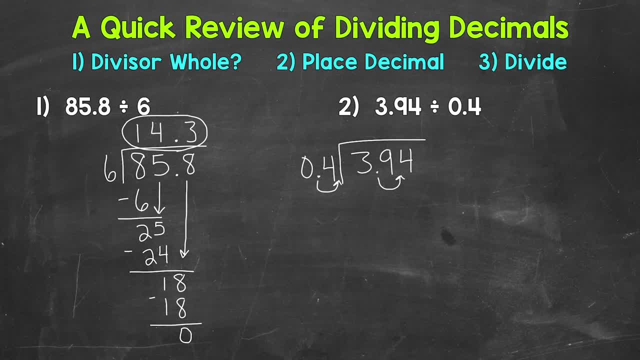 Once we get to this point We need to rewrite the problem with the whole divisor and the decimal placed. So we have 4 for our divisor And then 39 and 4 tenths for our dividend. Now is our divisor whole? Yes, 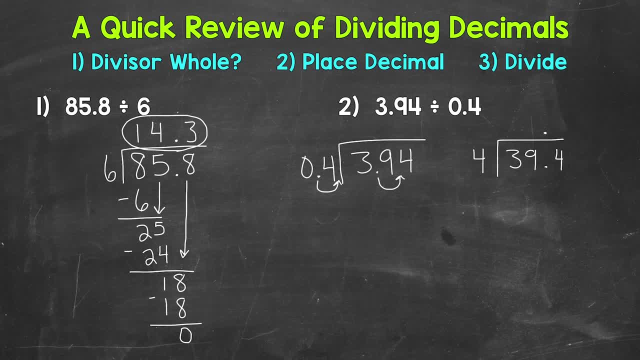 So we can bring our decimal straight up. Now it's placed where we need to have it in our answer And we can go through Our division process. Now we start with divide. So we have 3 divided by 4.. How many whole groups of 4 are in 3?? 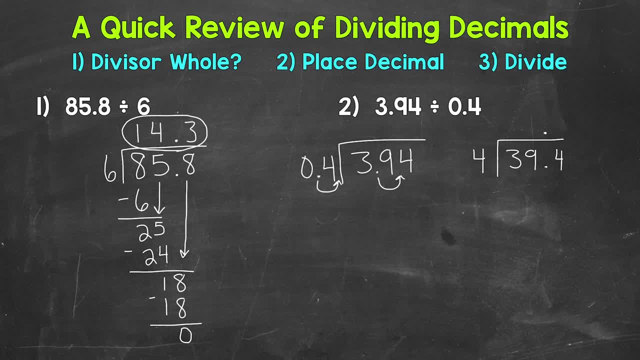 Well, we can't do that, So we need to move over and use that 9 as well And work with 39. So we have 39 divided by 4. How many whole groups of 4 are in 39?? Well, 9.. 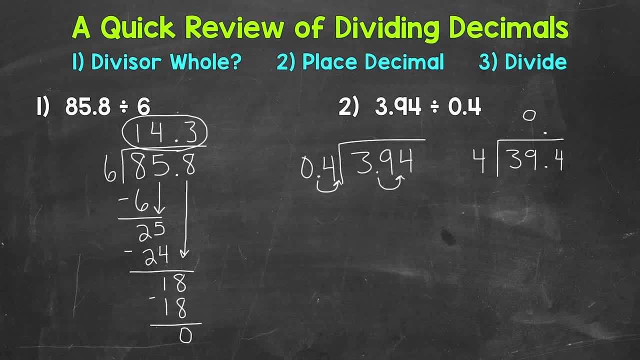 That gets us to 36.. So let's write this: 9 above the 39 there, Not above the 3. Make sure it goes above the 39. The 9 and 39. Because we used both of those digits for our divide step. 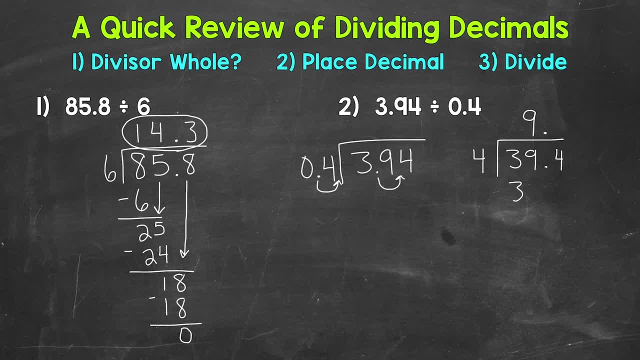 Now we multiply, So 9 times 4, 36, subtract, We get 3.. Then we bring down and repeat, So we have 34 divided by 4.. How many whole groups of 4 are in 34?? Well, 8.. 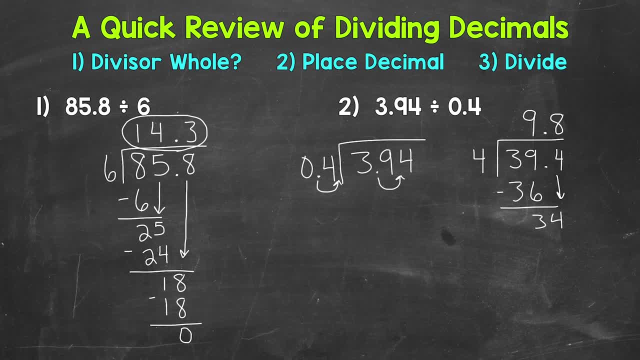 That gets us to 36.. So we have 34 divided by 4. That gets us to 32.. So 8 times 4, 32 subtract, We have 2.. Now we went all the way over to the furthest place to the right. 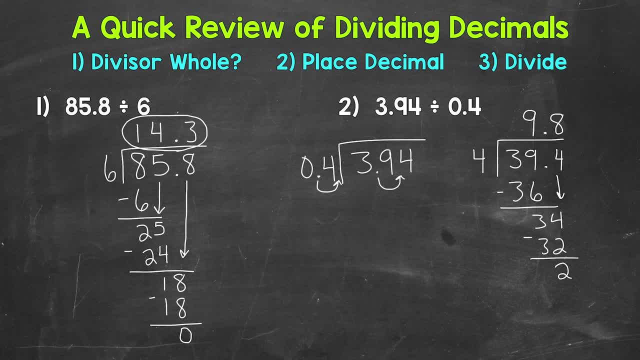 But we do not have a 0 at the end there once we subtracted. We do not want to put 9 and 8 tenths remainder 2.. We want to keep this in decimal form for the whole problem. So what we need to do, 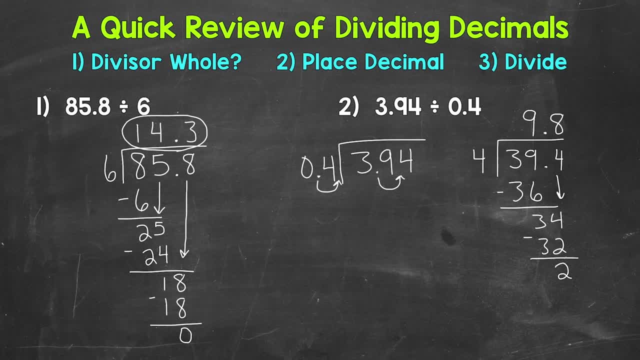 We need to work Until we get a clean cut 0 there at the end, And that's going to be our completed problem. So we need to put something on the end of this decimal to bring down and continue our process. So what can we put on the end of our decimal that will not change the value of that decimal? 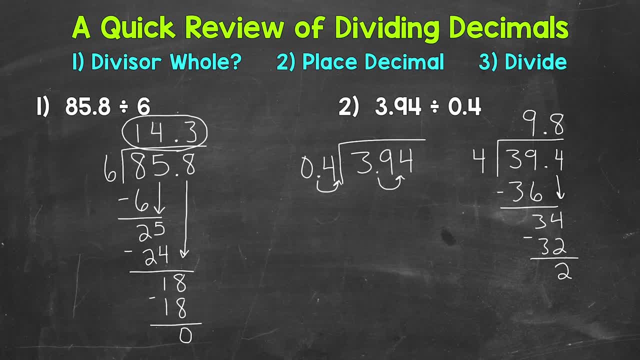 Well, a 0.. Remember, 0's to the right of a decimal do not change the value of that decimal. So we can use a 0 here and bring that down in order to continue our process. So we brought down the 0.. 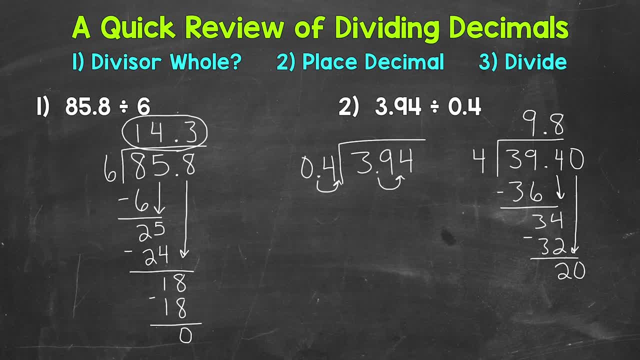 Now we repeat, We go back up to divide. So we have 20 divided by 4.. How many whole groups of 4 are in 20?? Well, 5.. That hits 20 exactly, And we can extend that bar there.